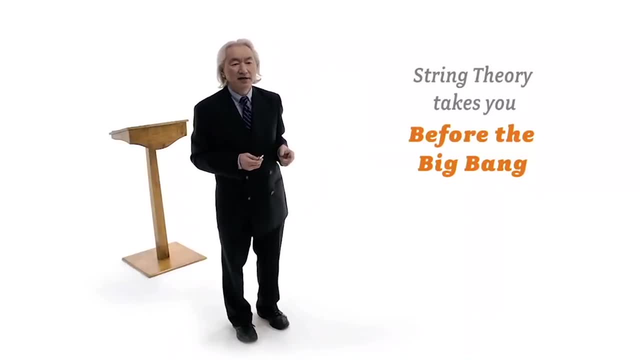 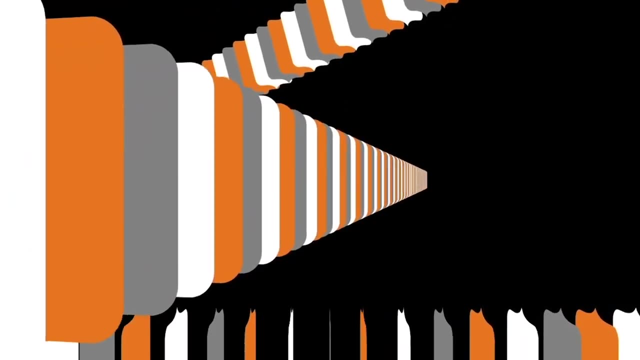 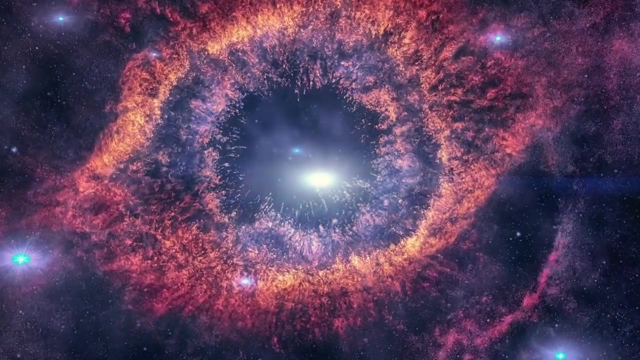 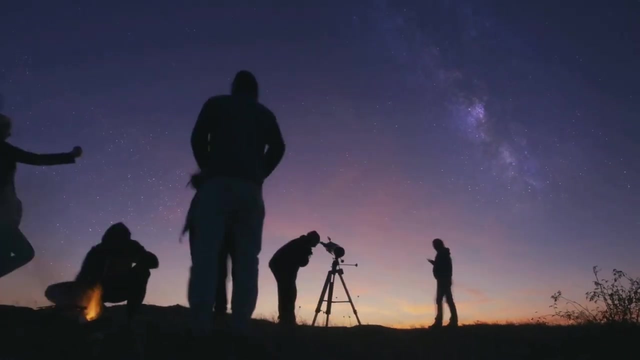 String theory takes you before the Big Bang, before Genesis itself. And what does string theory say? It says that there is a multiverse of universes. Have you ever wondered about the fascinating world of string theory? Join us on a journey to unravel the mysteries of the universe in this accessible video. String theory stands. 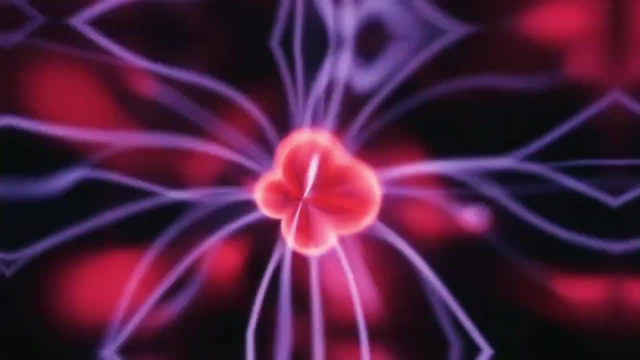 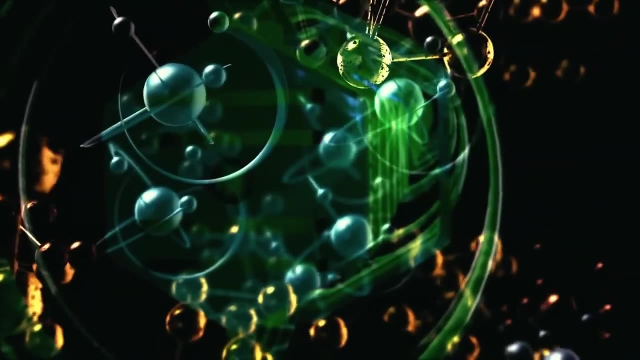 as one of the most ambitious and intriguing theories in the realm of theoretical physics. It seeks to provide a unified framework that can explain all the fundamental forces and particles in the universe. Originating in the late 20th century, string theory has captivated. 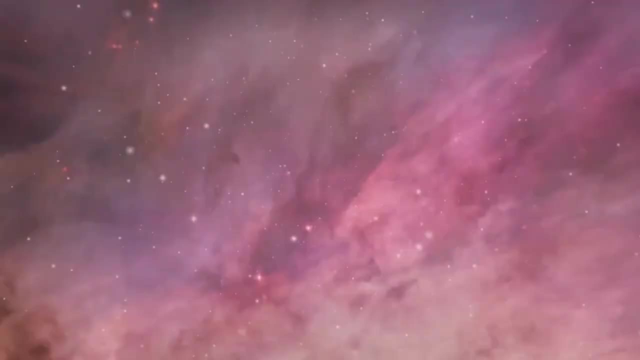 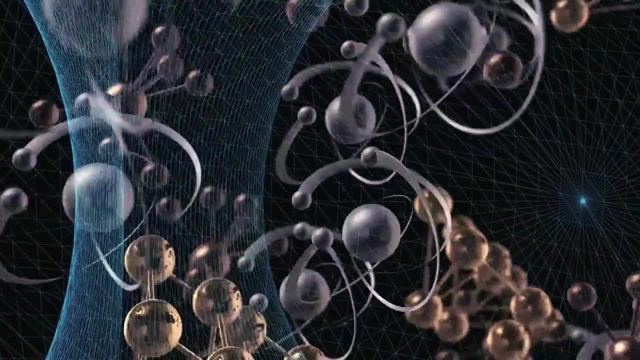 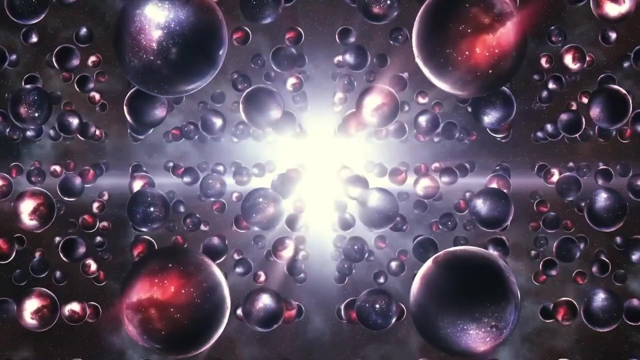 the minds of physicists, offering a new perspective on the fabric of reality itself: The Basics of String Theory. At its core, string theory posits that the fundamental building blocks of the universe are not particles like quarks or electrons, as conventional physics suggests, but rather tiny, one-dimensional strings. These strings, 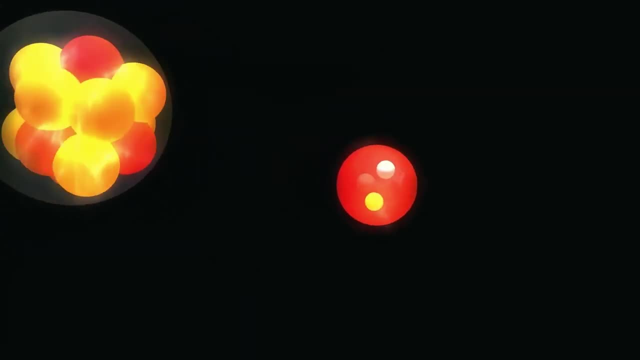 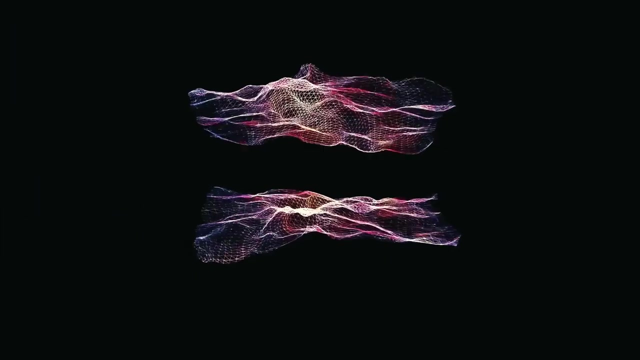 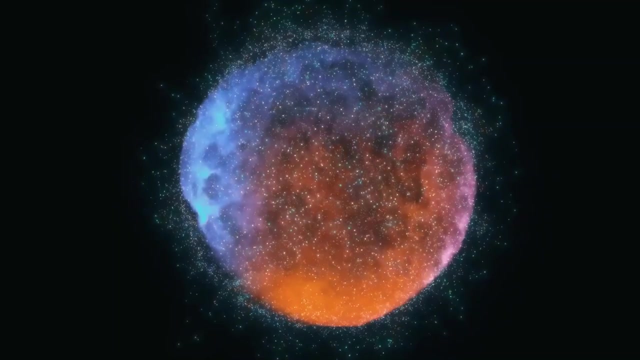 vibrate at different frequencies, and the various vibrational modes give rise to the diverse particles observed in the universe. The idea is that everything we perceive, from the smallest subatomic particle to the grandest galaxies, is composed of these vibrating strings, Unraveling the Basics of String Theory. String theory, a theoretical framework that 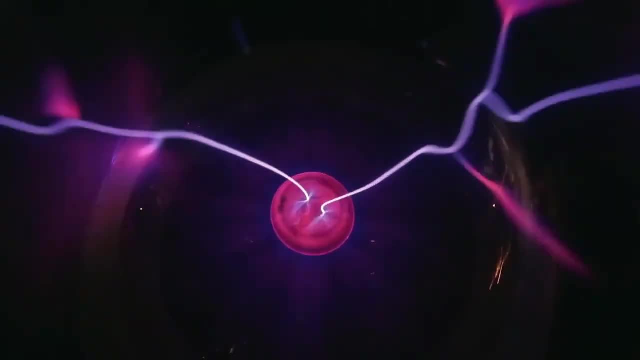 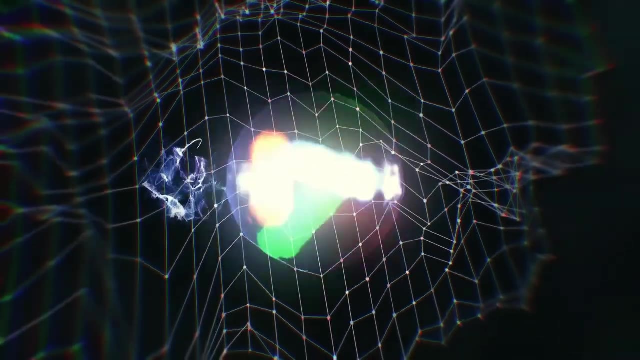 seeks to explain the fundamental nature of the universe is a a captivating and intricate concept that takes us beyond the realms of classical physics. In this exploration, we will break down the basics of string theory, aiming to make this complex topic accessible to enthusiasts of all levels. 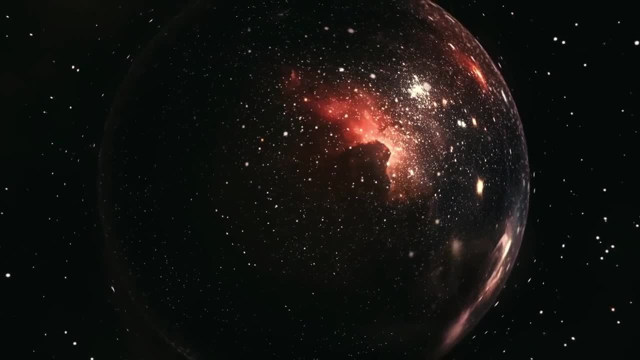 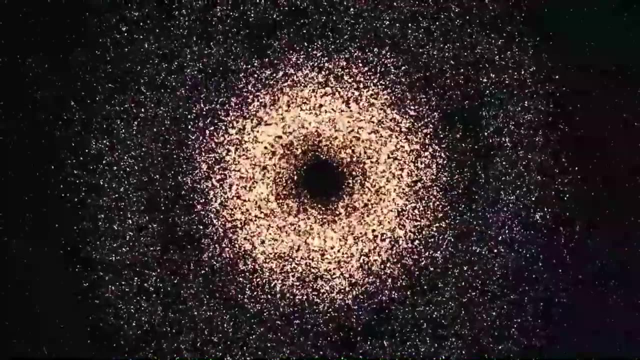 The Quest for Unity. At its core, string theory emerges from the quest for a unified theory of physics. In the early 20th century, physicists were confronted with the duality of quantum mechanics, governing the behavior of particles at the smallest scales, and general relativity. In the early 20th century, physicists were confronted with 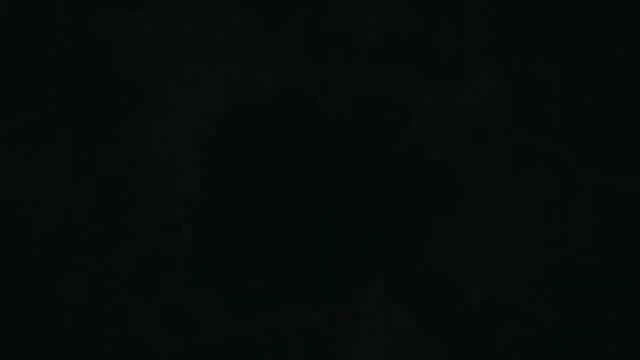 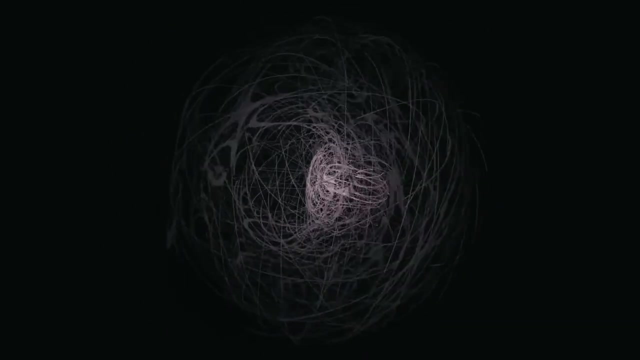 the duality of quantum mechanics governing the behavior of particles at the smallest scales, and general relativity, describing the force of gravity on cosmic scales. String theory strives to reconcile these two seemingly incompatible theories, offering a unified framework that encompasses both quantum mechanics and general relativity. 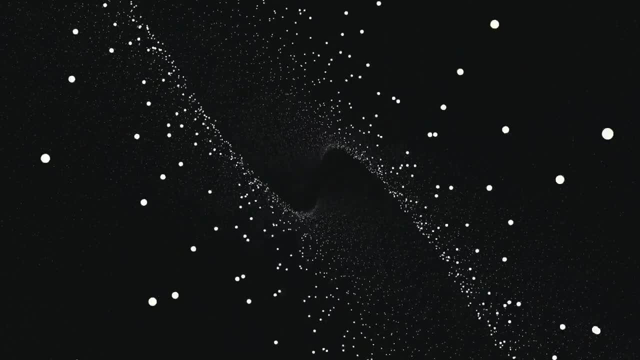 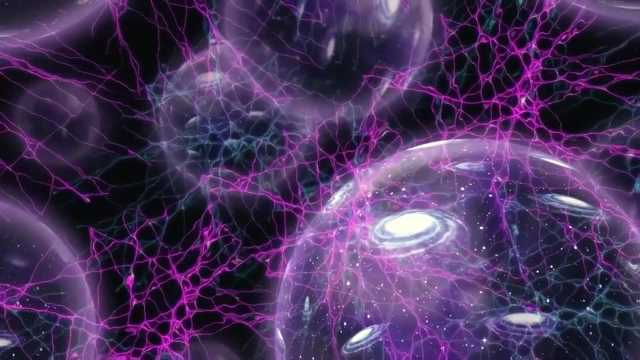 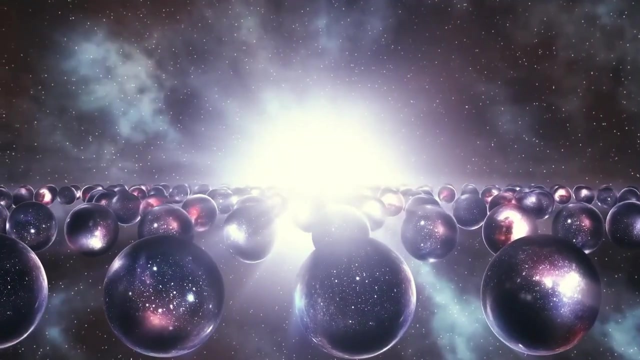 Strings as the Building Blocks. The foundational idea of string theory is elegantly simple, yet profound. Instead of imagining particles as point-like entities, string theory posits that the basic building blocks of the universe are tiny, one-dimensional space. These strings vibrate at different frequencies, akin to the strings of a musical. 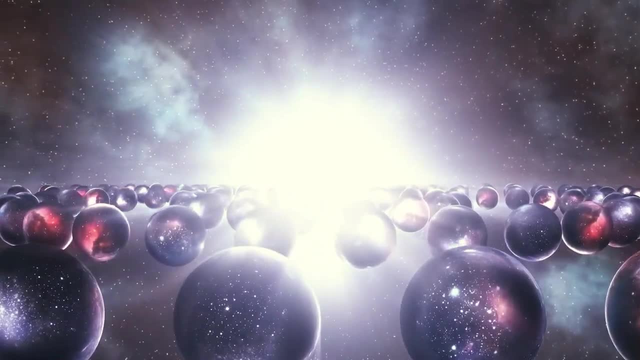 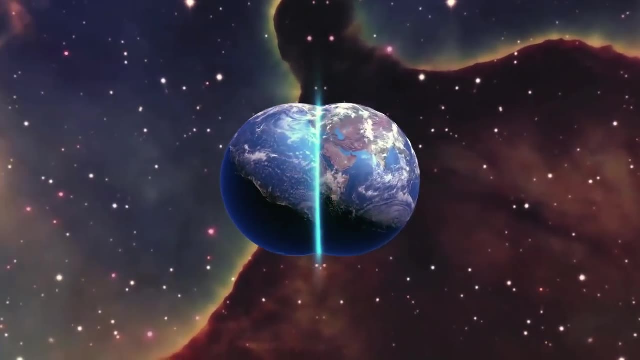 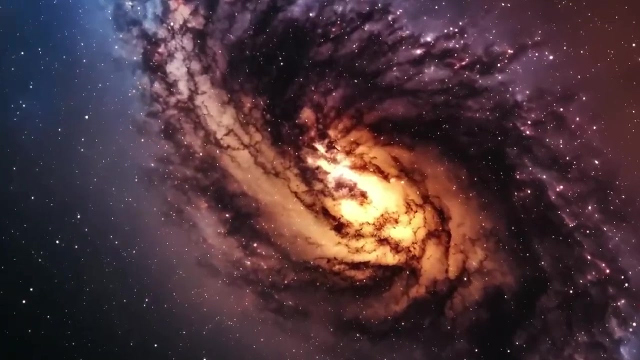 instrument producing the various particles observed in nature. The differences in vibration patterns give rise to the diverse particles that make up the fabric of our reality. Dimensions Beyond Three: In our everyday experience, we navigate a three-dimensional space. However, string theory introduces additional dimensions beyond the 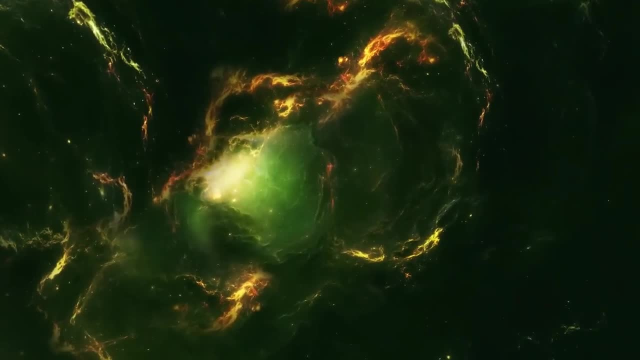 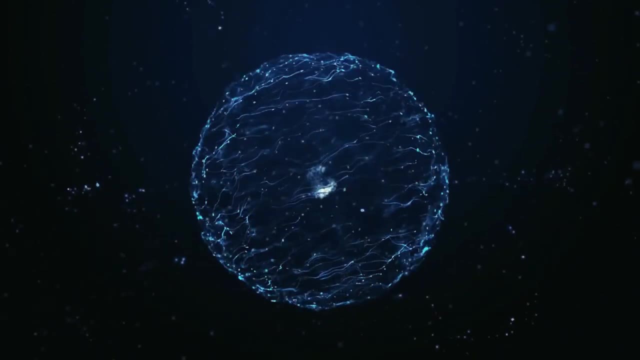 familiar three of length, width and height. These extra dimensions are compactified and they are tiny and curled up, making them imperceptible at our macroscopic stale. Understanding these extra dimensions is crucial to comprehending the intricacies of string theory and its implications. 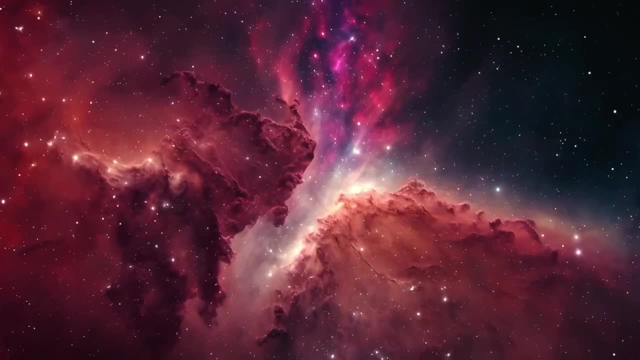 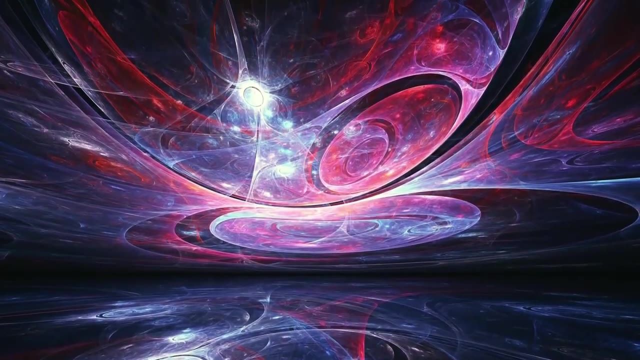 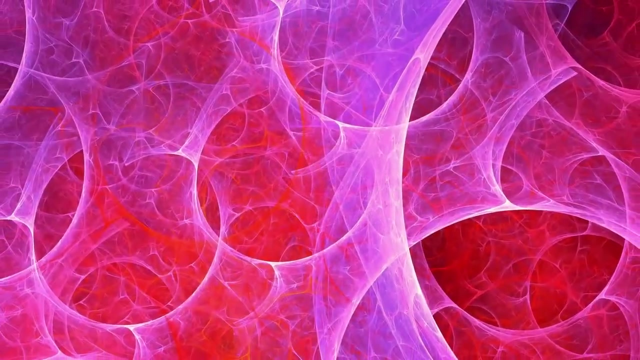 for the structure of the universe: Quantum Mechanics and General Relativity Unveiled. One of the key challenges in theoretical physics has been reconciling the principles of quantum mechanics and general relativity. Quantum mechanics successfully describes the behavior of particles at the quantum level, while general 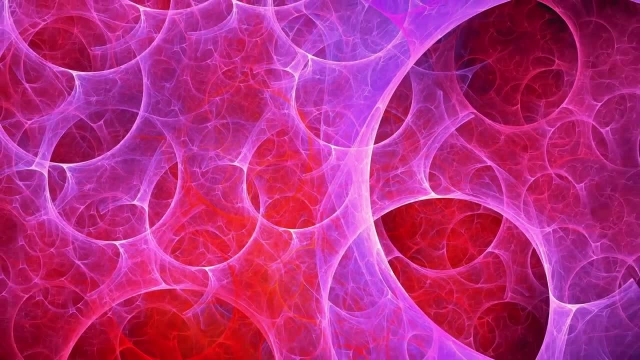 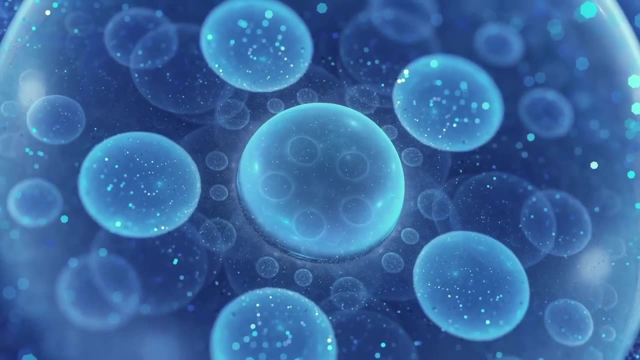 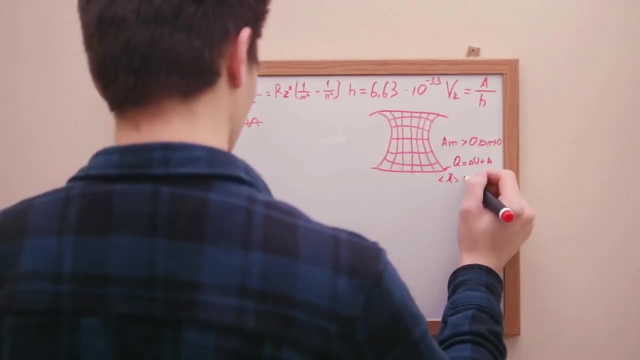 relativity explains the force of gravity on cosmic scales. String theory offers a potential solution by providing a framework that seamlessly incorporates both quantum mechanics and general relativity, creating a harmonious description of the universe. The Vibrating Symphony of Strings. Imagine the universe as a grand orchestra with 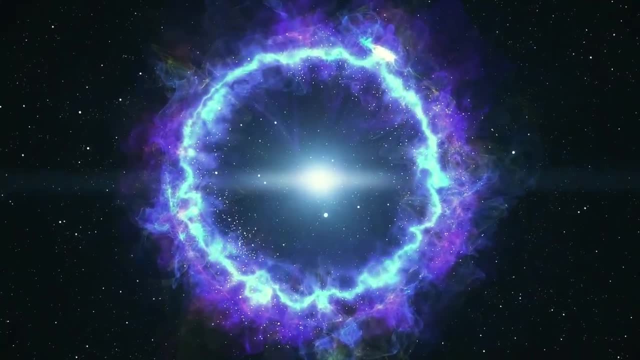 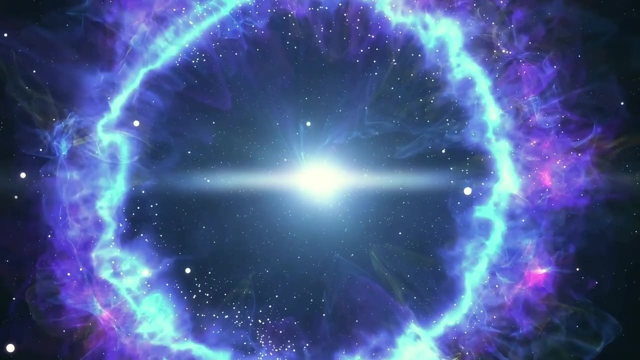 each particle playing a unique note in a cosmic symphony. In string theory, these particles are the result of the vibrations of fundamental strings. The variety of particles, from quarks to electrons, emerges from the different harmonics produced by the vibrating strings. This 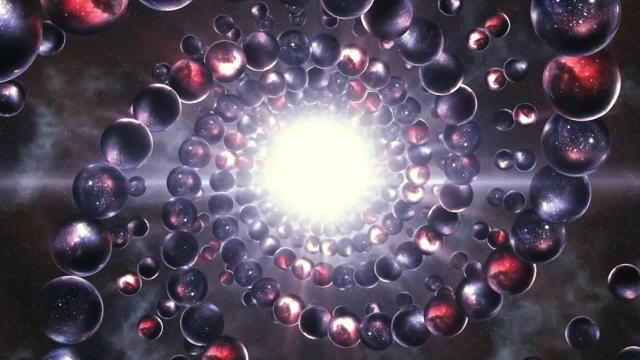 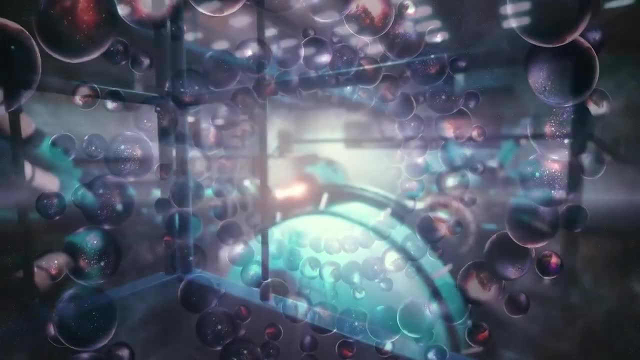 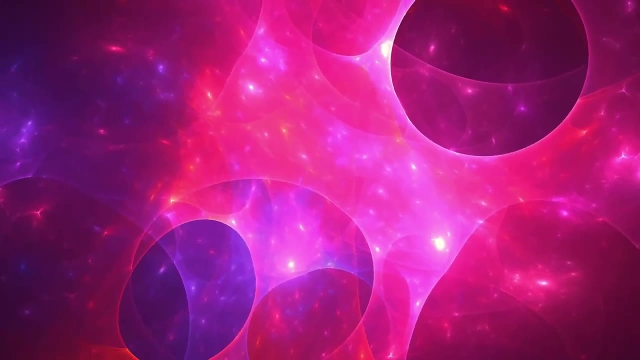 elegant concept provides a unified explanation for the diverse array of particles observed in particle physics experiments, Extra Dimensions and Hidden Realms. The introduction of extra dimensions in string theory adds a layer of complexity to our understanding of the universe. While we perceive only three spatial dimensions, string theory suggests the existence of extra dimensions that play 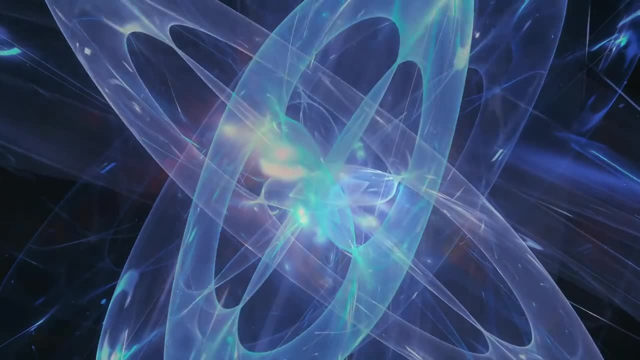 a crucial role in shaping the properties of the universe. In string theory, the existence of extra dimensions plays a crucial role in shaping the properties of the universe. String theory suggests the existence of extra dimensions that play a crucial role in shaping the properties of particles and forces. These extra dimensions, though elusive, hold the key to unraveling. 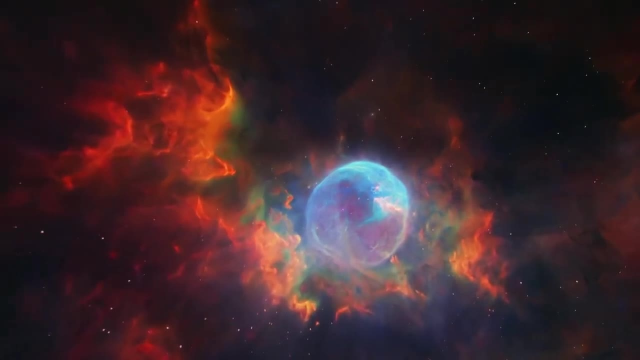 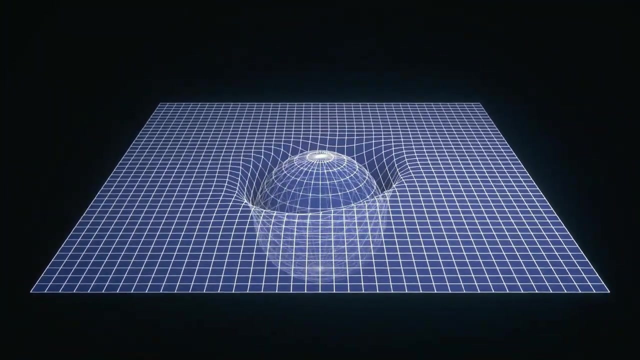 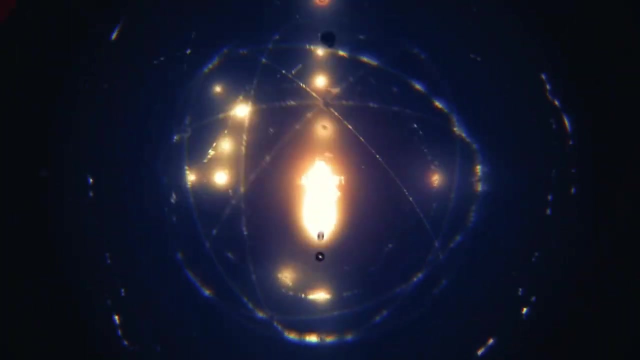 mysteries that classical physics cannot address: Challenges in Experimental Validation. One of the distinctive features of string theory is the lack of direct experimental evidence. Unlike many scientific theories that can be tested through empirical observations, string theory remains largely theoretical. Physicists are faced with the challenge of devising experiments or observations that 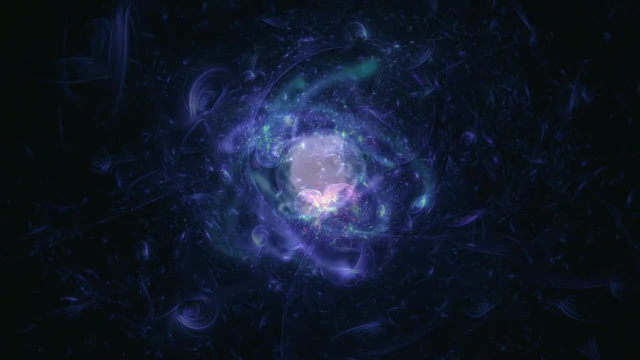 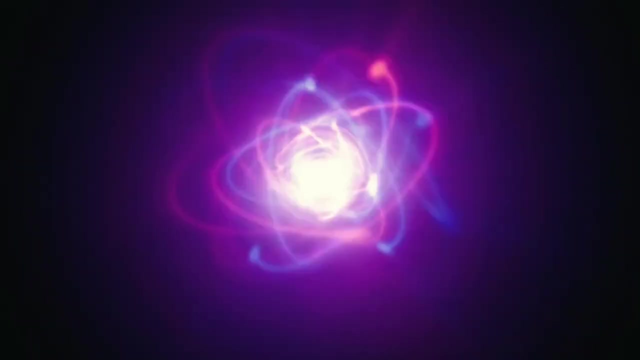 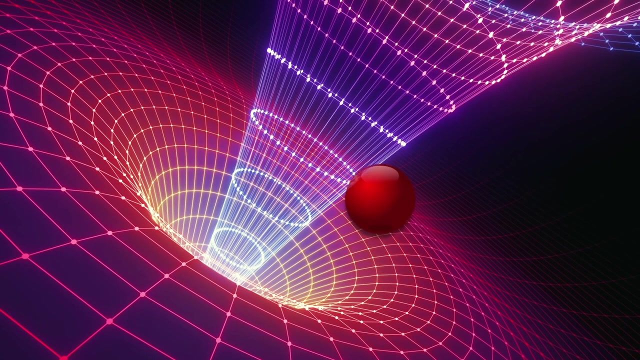 could provide evidence for the existence of strings. This quest for experimental validation is ongoing, with researchers exploring avenues ranging from high-energy particle accelerators to cosmological observations. Implications for the Nature of Gravity. String theory has profound implications for our understanding of gravity. Unlike in classical physics, where gravity is described as the 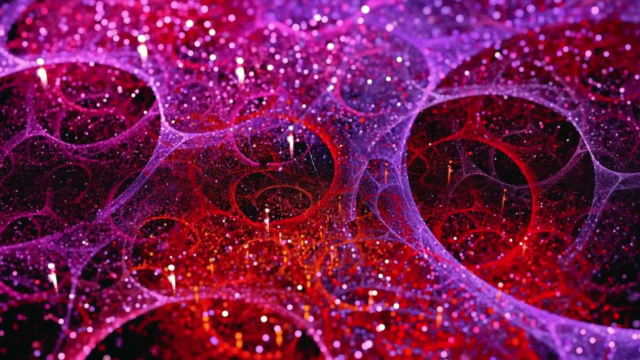 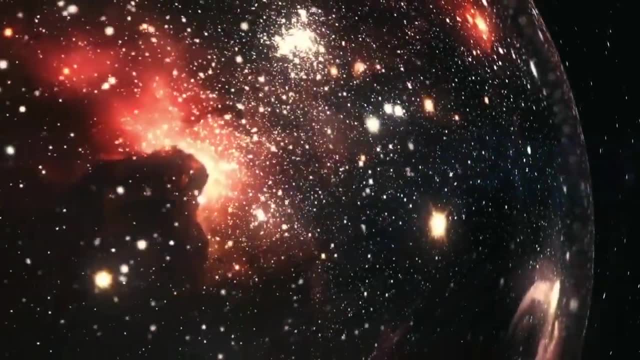 curvature of spacetime. string theory suggests that gravity is mediated by the exchange of particles called gravitons. String theory has profound implications for our understanding of gravity. This novel perspective on gravity opens up new avenues for exploring the fundamental nature of the gravitational force and its role in the cosmos. 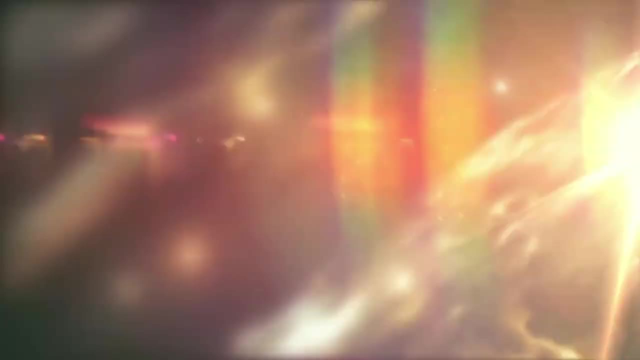 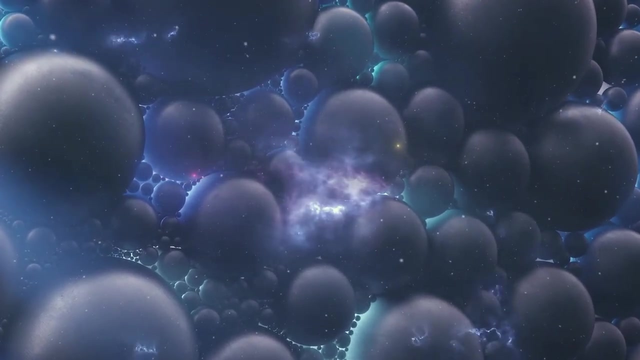 Parallel Universes and Multiverse Hypotheses. As string theory delves into the nature of extra dimensions, it also gives rise to intriguing possibilities, such as the existence of parallel universes. Some variations of string theory propose a multiverse where our universe is. 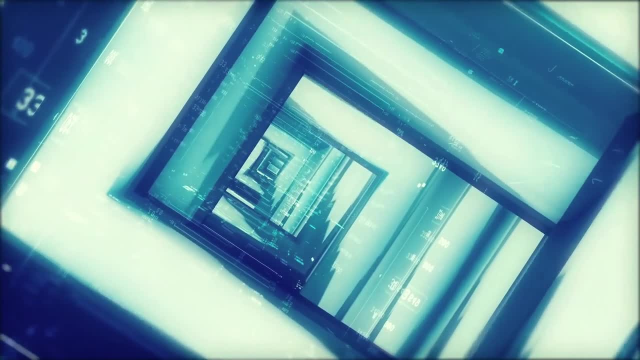 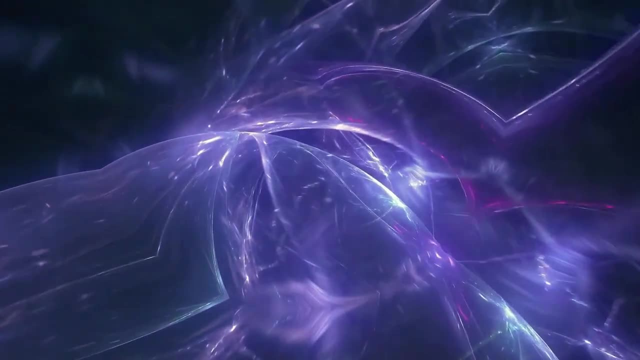 just one of many, each with its own unique properties. String theory is a theory of the universe where the universe is just one of many, each with its own unique properties. While speculative, these ideas highlight the profound implications that string theory may have on our conception of reality. 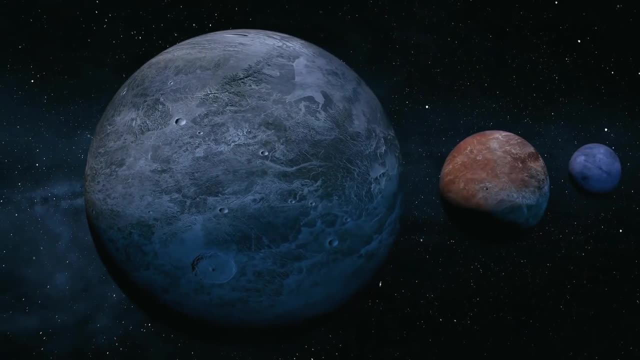 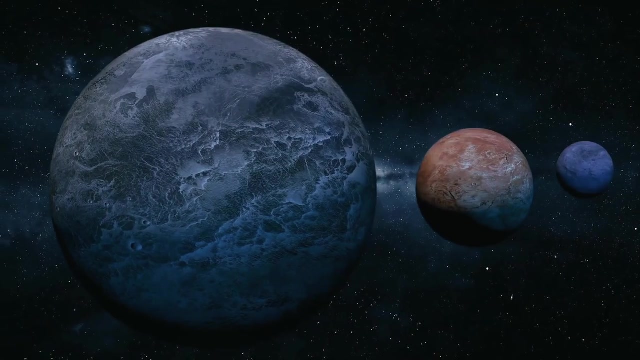 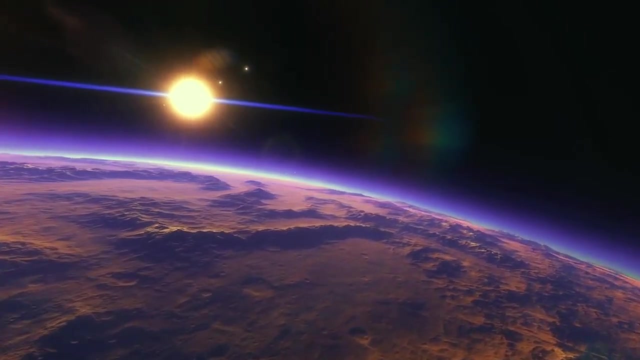 The Road Ahead String theory, despite its theoretical elegance, remains a work in progress. The quest to fully understand and validate its predictions continues to be a driving force in theoretical physics. As technology advances and our understanding of the cosmos deepens, researchers hope to find experimental evidence that either supports: 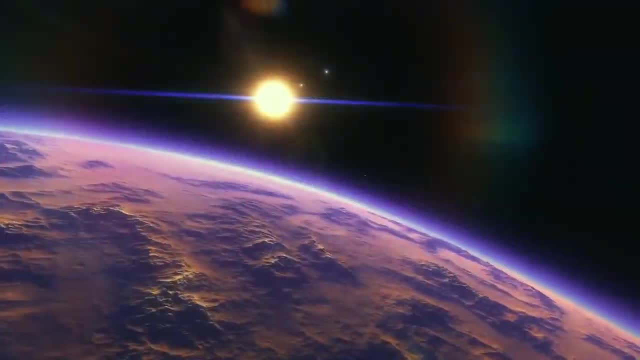 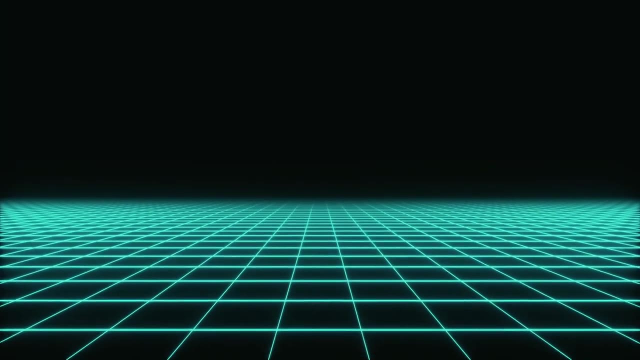 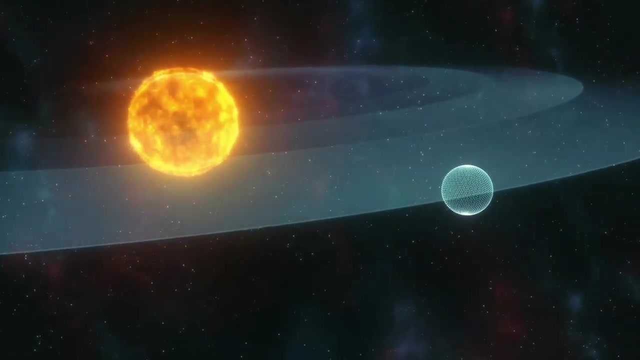 or refutes the tenets of string theory. The journey into the microscopic fabric of the universe is ongoing, with each discovery and breakthrough bringing us closer to unraveling the mysteries encapsulated in the vibrating strings that underlie our reality. Exploring the Implications and Challenges of String Theory. In this exploration, we delve into the profound implications string theory has on our conception of the cosmos, while also addressing the formidable challenges that researchers face in unraveling its mysteries. Gravity Reimagined: One of the primary implications of string theory is the reimagining of gravity In classical 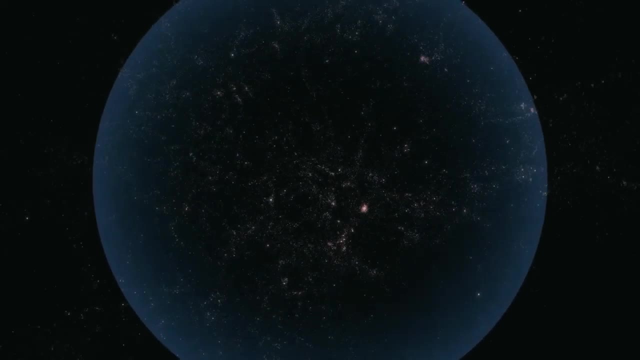 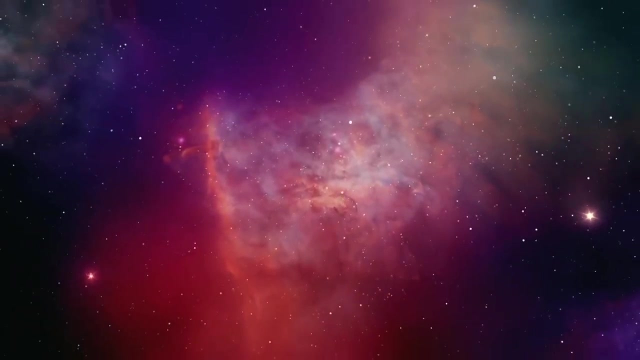 physics, gravity is described by general relativity as the bending of spacetime caused by mass. However, string theory introduces the concept of gravitons, hypothetical particles that mediate the force of gravity. This shift in perspective not only unifies gravity with 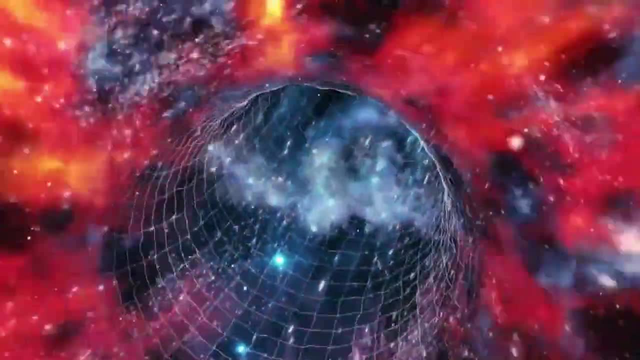 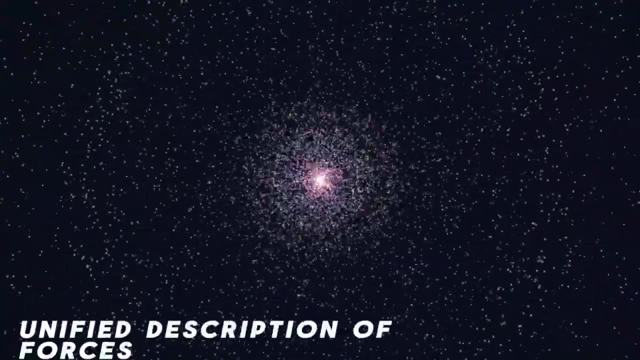 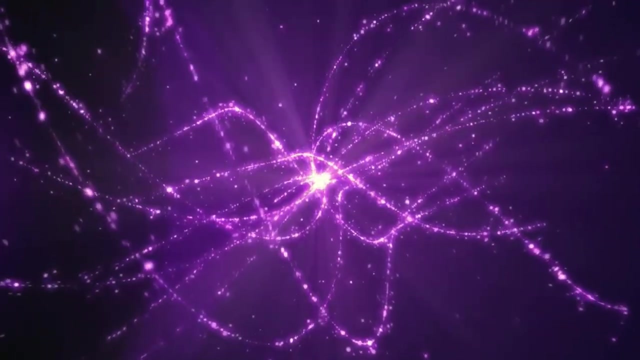 the other fundamental forces, but also opens new avenues for investigating the nature of gravitational interactions at both quantum and cosmic scales. Unified Description of Forces. String theory seeks to achieve a unified description of the fundamental forces in the universe, bringing together electromagnetism, the strong nuclear force, the weak nuclear force and 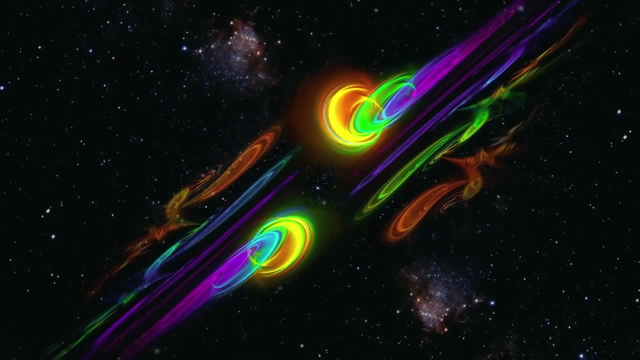 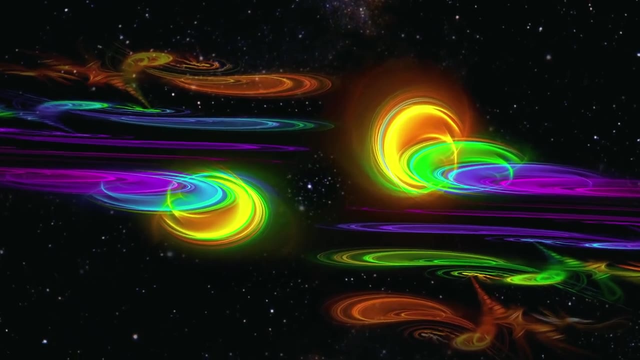 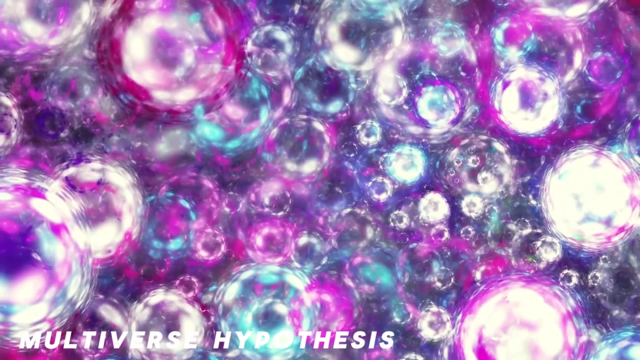 gravity. By attributing these forces to the interactions of vibrating strings, string theory offers a tantalizing vision of a single cohesive framework governing the diverse phenomenon observed in the cosmos. String Theory promises a deeper understanding of the fundamental nature of reality. Multiverse Hypotheses: The idea of a multiverse is a captivating implication of string theory. Some variations of the theory propose the existence of multiple universes, each with its own set of physical constants and properties. These parallel universes could exist in different dimensions or with different compactifications of extra dimensions, introducing a vast cosmic landscape beyond our observable universe. While speculative, 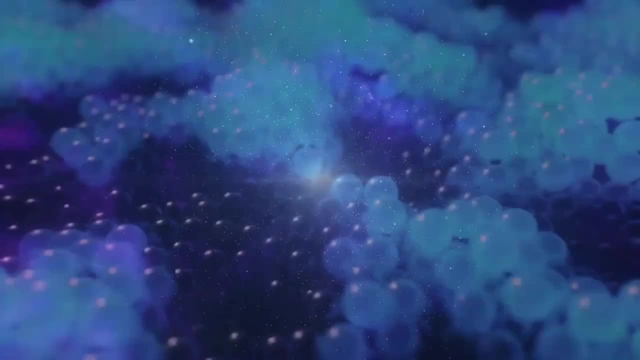 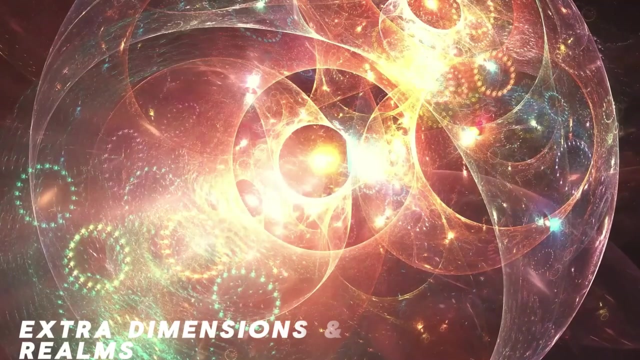 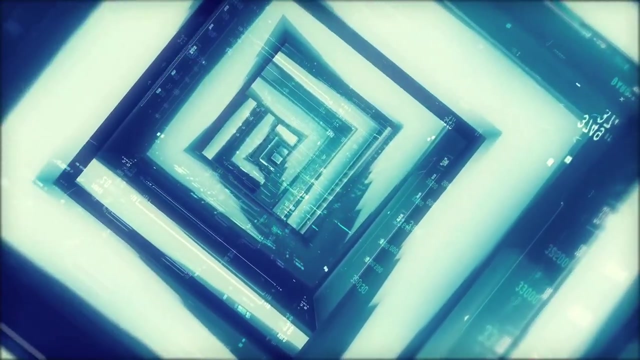 the multiverse hypothesis arises naturally from certain formulations of string theory, prompting researchers to explore the potential implications for the broader structure of the cosmos, Extra Dimensions and Hidden Realms. String theory necessitates the inclusion of extra dimensions beyond the three spatial dimensions we perceive in our everyday experiences. These extra dimensions play a crucial role. 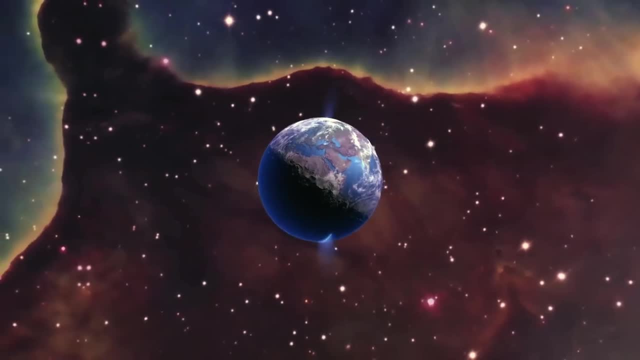 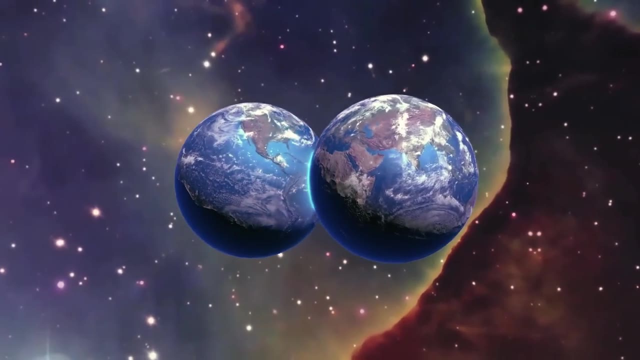 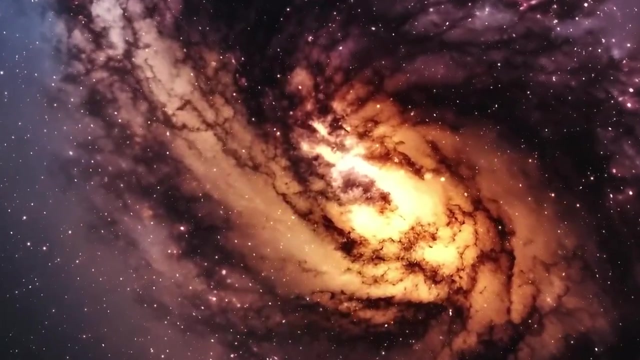 in shaping the properties of particles and forces in ways that classical physics cannot explain. The challenge lies in understanding the nature of these extra dimensions, their size and their impact on observable phenomena. If successfully unraveled, these hidden realms could provide insights into the mysteries of dark matter, dark energy and other cosmic enigmas. 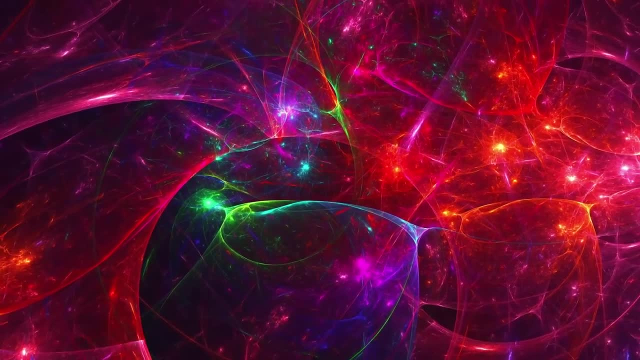 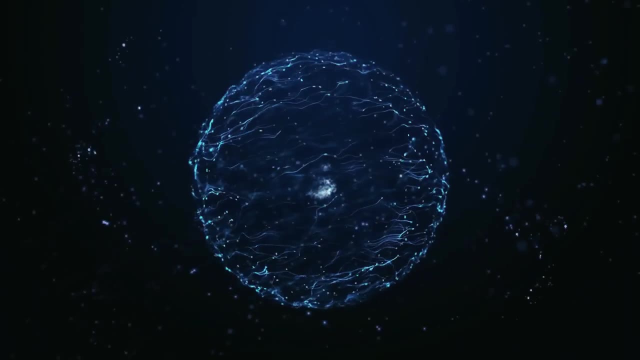 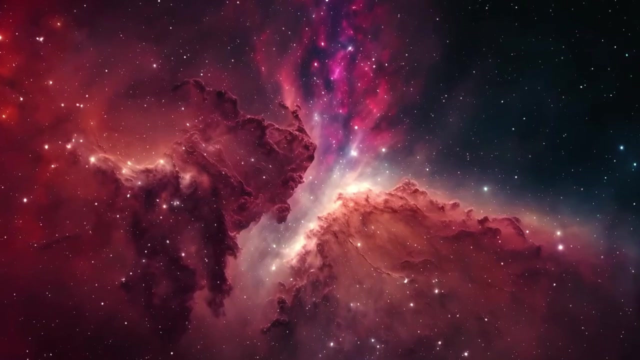 Quantum Entanglement and Non-Locality. String theory introduces a novel perspective on quantum entanglement, the phenomenon where particles become interconnected in such a way that the state of one particle instantaneously influences the state of another, regardless of the distance between them. The theory suggests that entanglement might be a consequence of the intricate relationships between vibrating strings, implying a deeper connection between seemingly separate entities in the quantum realm. This raises questions about the nature of nonlocality and the fundamental interconnectedness of all things in a string-theoretic framework. 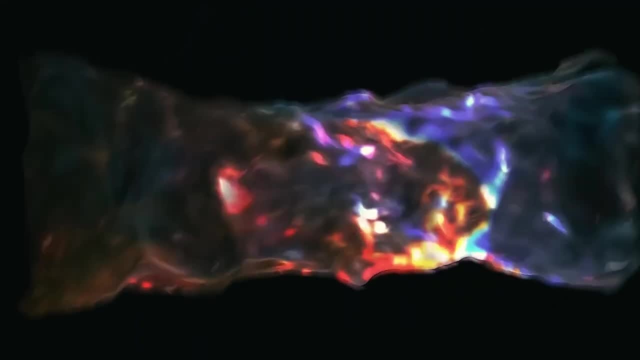 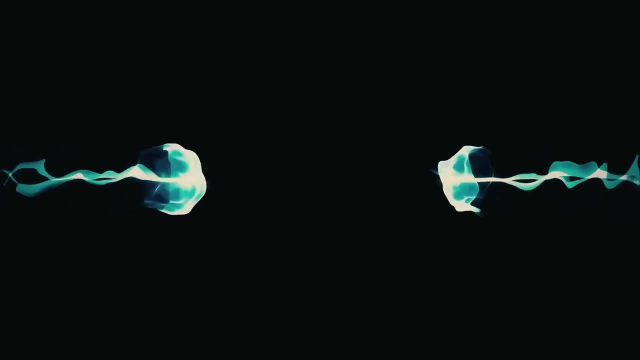 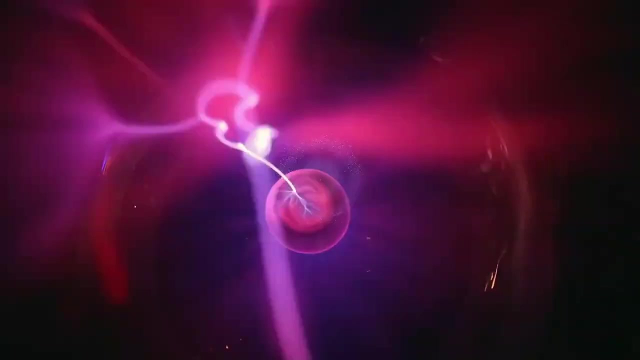 Challenges in Experimental Validation. Despite its theoretical elegance, string theory faces significant challenges in terms of experimental validation. Unlike many scientific theories that can be tested through direct observation or experimentation, the scale at which strings vibrate is currently beyond the reach of our experimental capabilities. 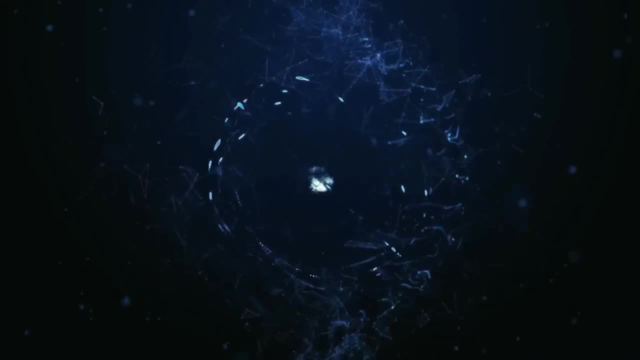 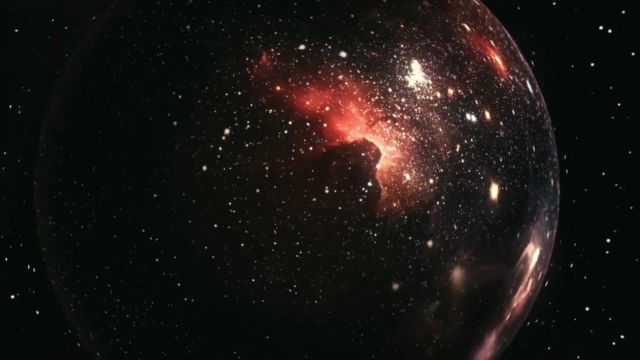 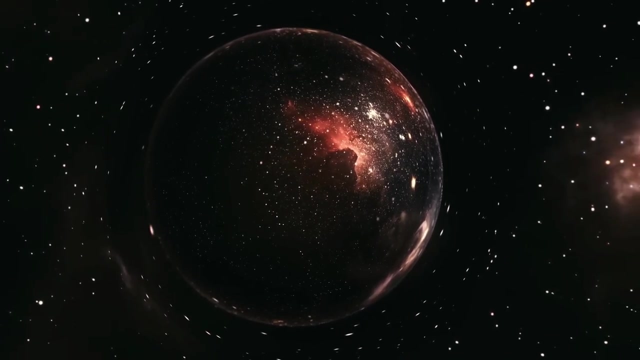 The minuscule size of strings, estimated to be on the order of the Planck length, poses a formidable challenge for experimental physicists. Researchers are exploring innovative approaches, such as high-energy particle accelerators and cosmological observations, to indirectly detect signatures of string-like behavior. 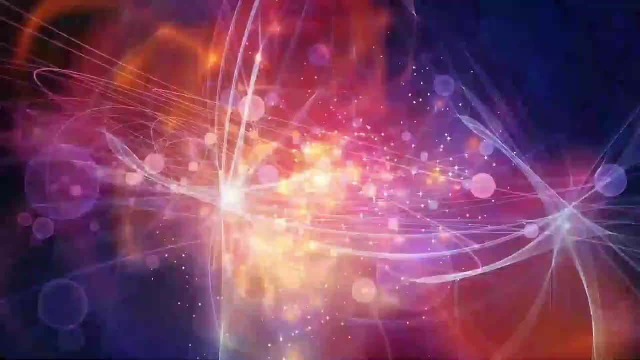 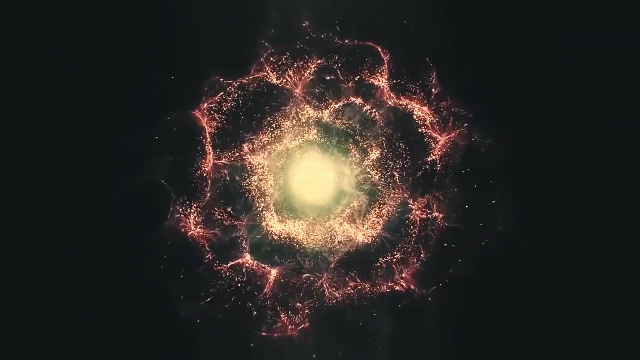 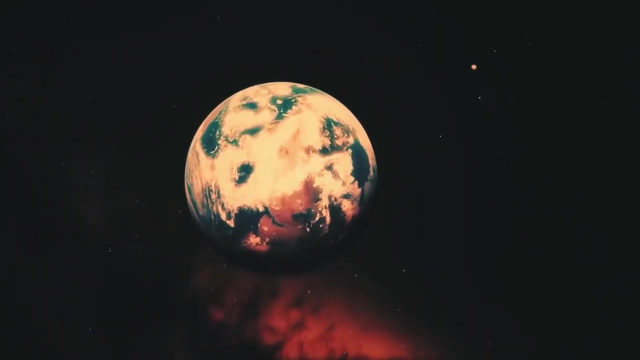 in the hope of providing experimental support for string theory. Landscape of Possibilities. The multiverse hypothesis, a natural consequence of certain formulations of string theory, introduces a vast landscape of possibilities, each with its own set of physical laws. Navigating this landscape raises. 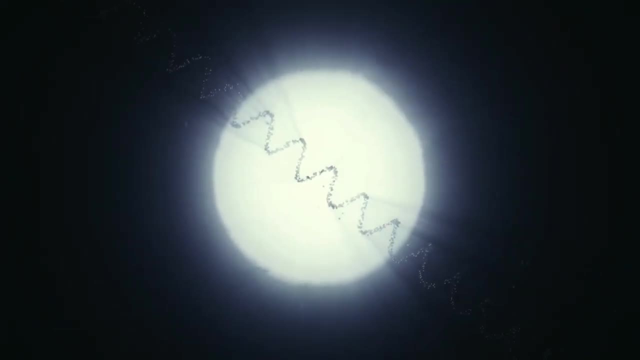 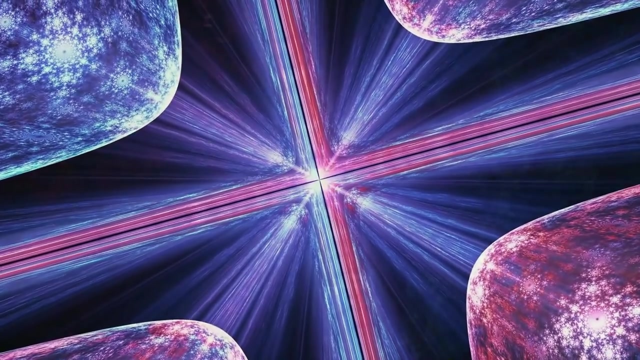 questions about the uniqueness of our universe. The theory suggests that string theory is a concept that is based on the fundamental constants and the predictability of its fundamental constants. Understanding the implications of a multiverse requires grappling with the concept of the Anthropic Principle, which suggests that the fundamental constants of our universe 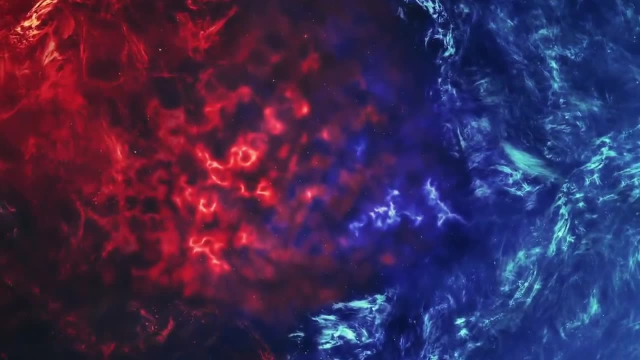 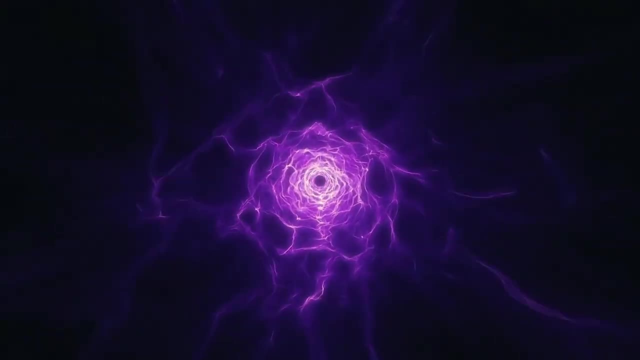 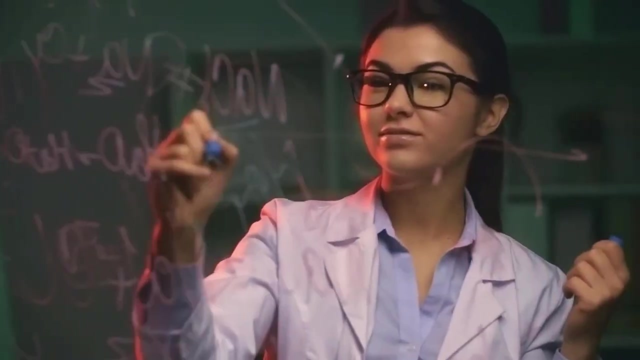 might be finely tuned to allow for the existence of life. String theory in this context prompts us to explore the broader implications of a cosmic landscape teaming with diverse universes. Unification of Mathematics and Physics: String theory has deepened the connection between mathematics and physics. The elegance and mathematical beauty of the theory have led 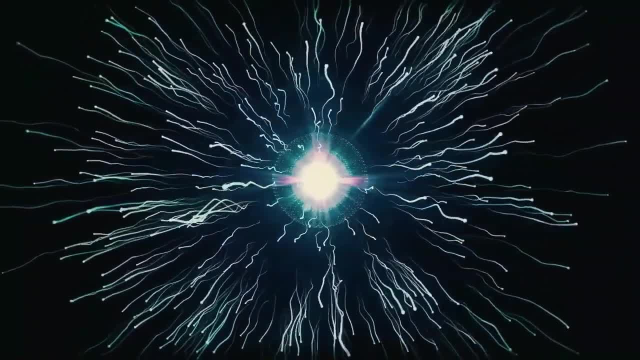 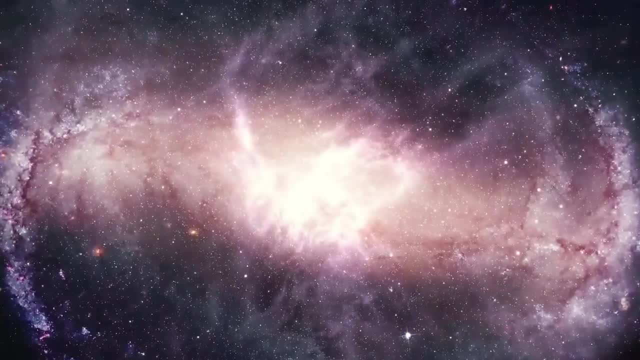 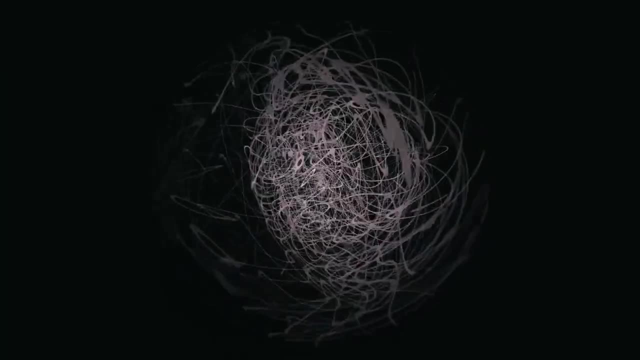 physicists to explore advanced mathematical concepts, including geometry and topology, in the quest to understand the fundamental nature of the universe. The interplay between abstract mathematical structures and physical reality is a hallmark of string theory, challenging researchers to push the boundaries of both disciplines: accessibility and communicating. 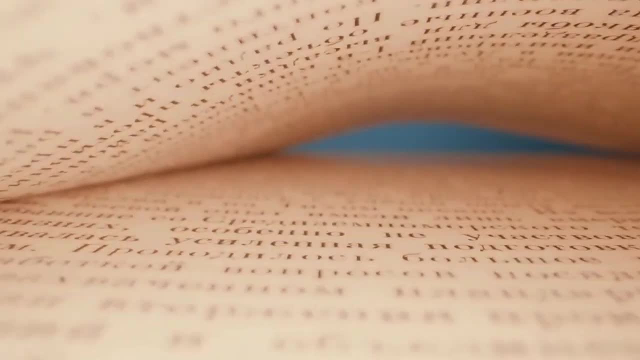 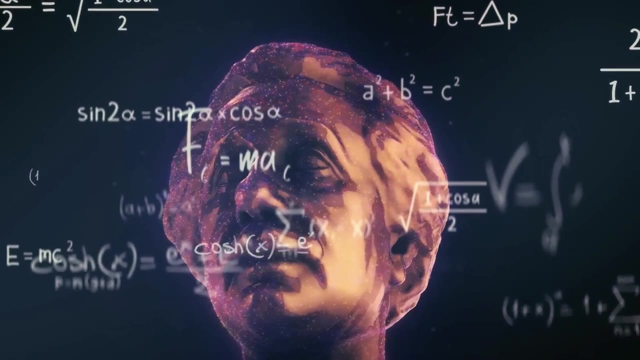 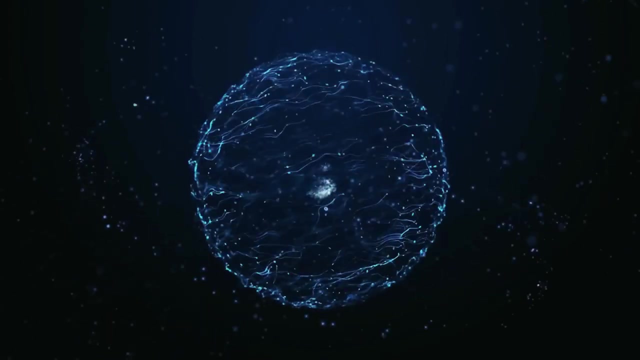 complexity. A challenge inherent in string theory lies in its complexity and abstract nature. Communicating these complex ideas to a broader audience, including students and the general public, requires innovative educational approaches. Researchers must bridge the gap between the intricate mathematical formalism of string theory and accessible explanations that convey the essence.